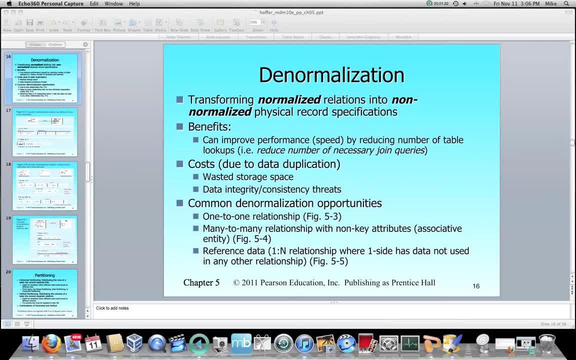 So there are four tables, all of which have to be joined together. So that's going to be. That's going to require some performance. That's going to be a performance hit to join all of those tables together. There is a cost associated with denormalization, in that now I have duplicated data right, So now I'm going to be storing data. 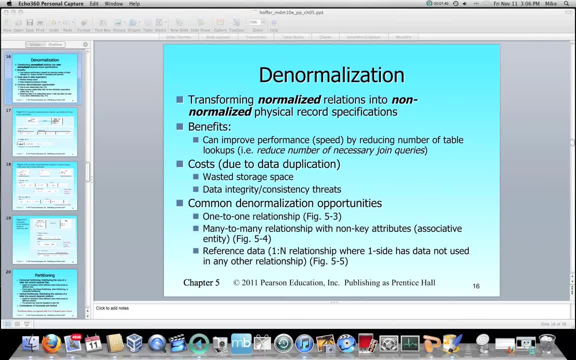 We're going to be storing data in a fashion that is against normalization, hence the word denormalization. So I'm going to have wasted storage space And since I'm doing this, I'm going to set myself up for the possibility Of data integrity problems. right, I can have update anomalies and insert anomalies and deletion anomalies. 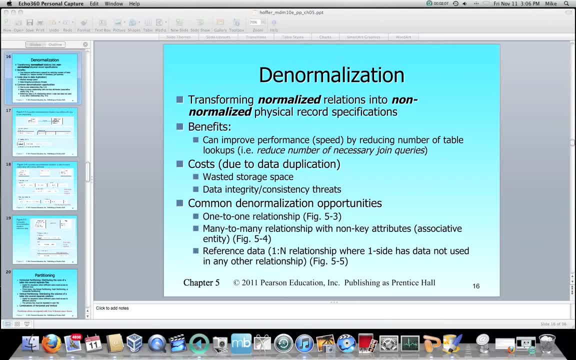 And that's a cost, because I'm going to have to put something in place to keep that in place. all right, to keep the data consistent, When we talk about denormalization, there are usually opportunities for that And we're going to go through. 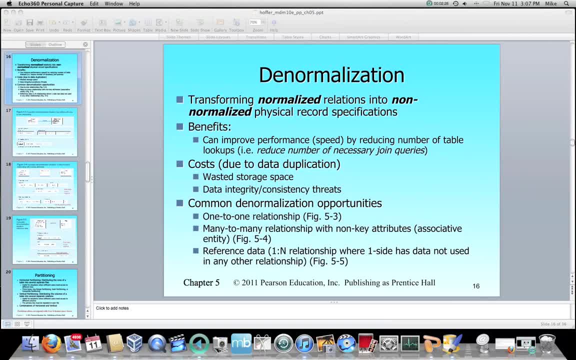 A couple of these opportunities. if we have one to one relationships, in other words, if we have super type subtypes, for instance, we have one to one relationships, That's, that's a an area where we can consolidate our data and denormalize. 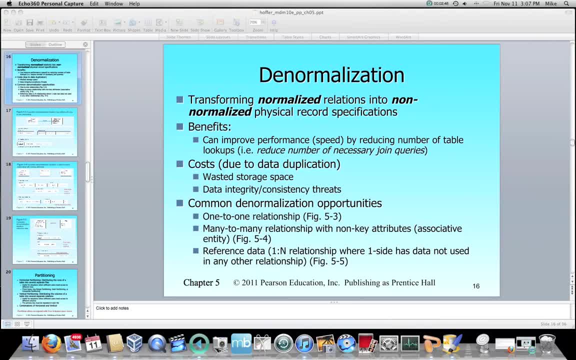 We have many, to many, relationships with non key attributes, right Associated entities, And we'll go through an example of that And we can have reference data. We'll Where one side has data not used in any other relationship- right, And that's what we talk about. 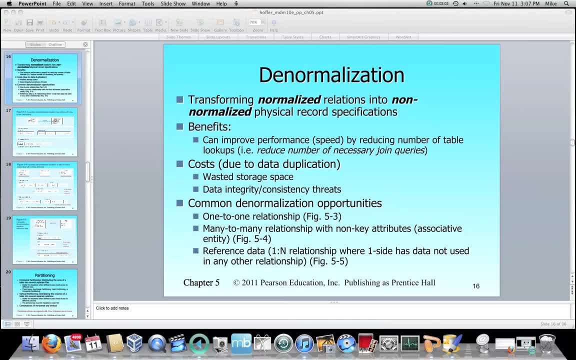 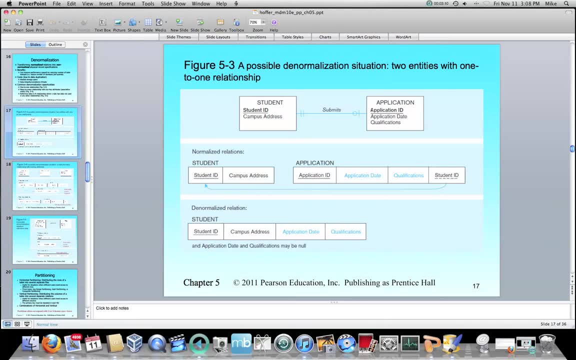 Look up stuff. So let's go through some of the examples. So here we have a one to one right, So a student will submit an application And if a student submits an application of so we have our ERD right And then that gets into. we change that into the relational model. 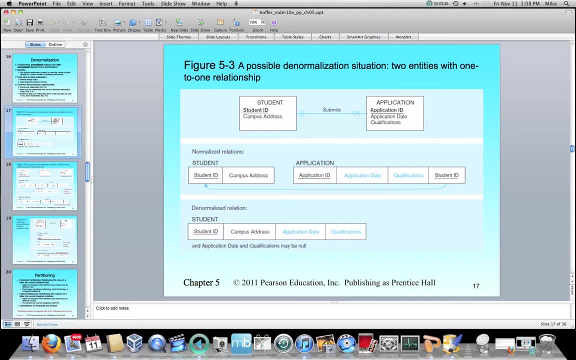 So we have normalized relations And we see that the student ID becomes a foreign key in the application right Then what we can do is, instead of storing that application ID- the foreign key of the student ID- in the application table, we will merge them together so that we have this. the student table now keeps track of the application data and the qualifications.